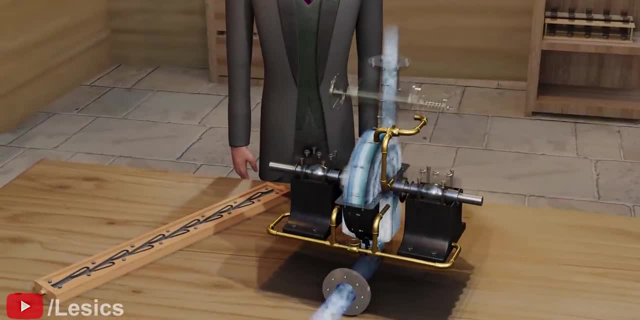 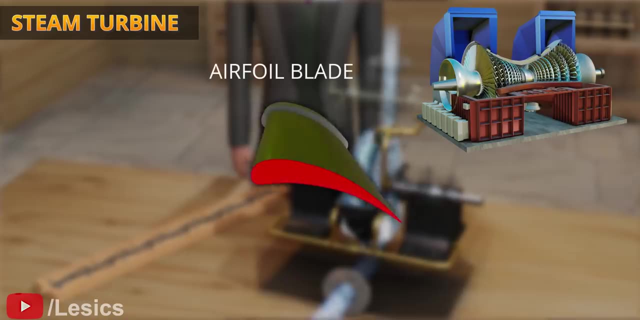 to understand this interesting piece of technology and, towards the end, we will also verify Tesla's efficiency claim. Modern day turbines work on the airfoil principle. You can see the fluid gushing over the airfoil cross-section will generate lift force on it and the airfoil will be used to generate lift force on the turbine. 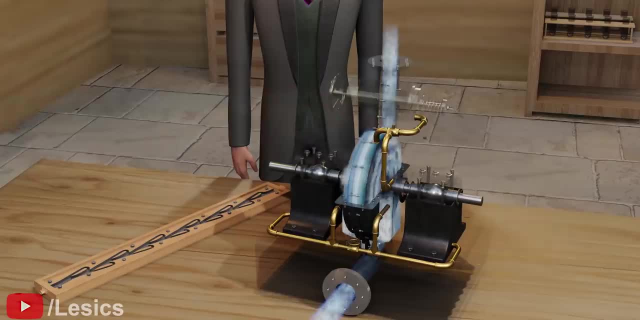 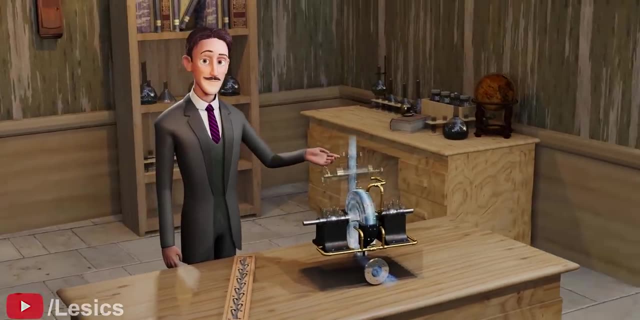 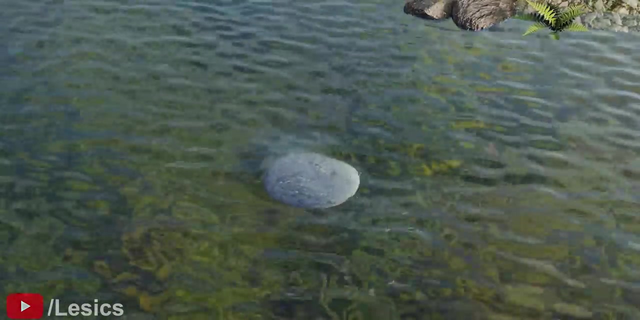 And make the blade turn. However, to make this turbine spin, Nikola Tesla relied on a totally different phenomenon: the viscous effect of fluid on solid surfaces. You might have seen this effect before. When water flows over a rounded stone, it makes the stone move because of the viscous force between the water and the stone surface. 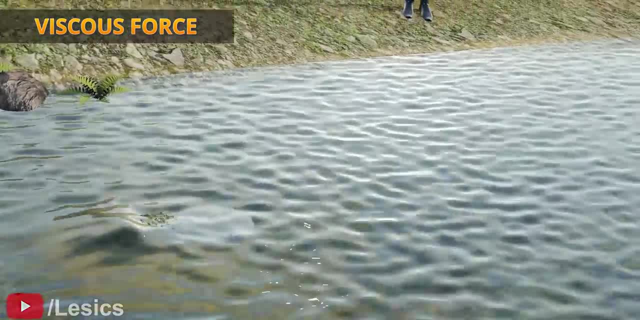 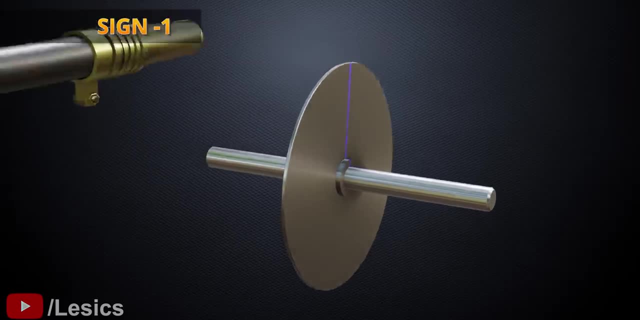 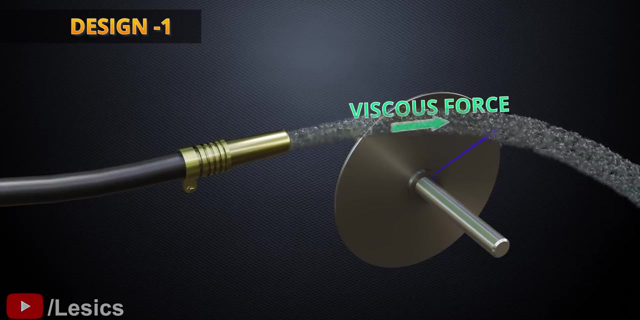 Nikola Tesla extrapolated this very force to run his turbine. Who knows, Tesla might have got inspiration for his turbine from this very example. If you produce the viscous force tangential to a disc, it will start to spin. Hooray, you have produced the simplest form. 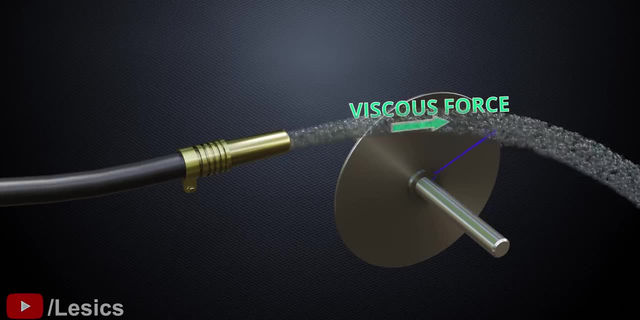 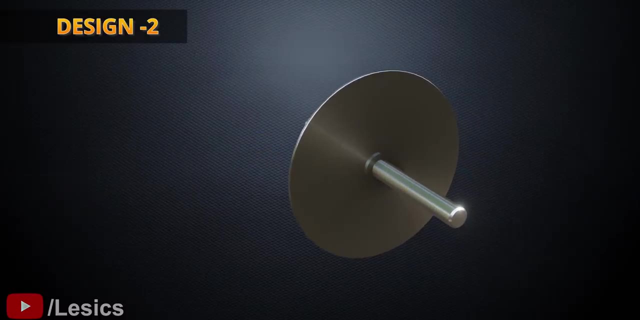 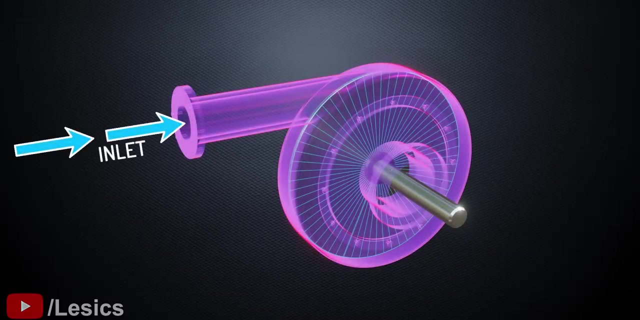 of Tesla turbine. However, this is quite an inefficient turbine. Most of the jet's energy is lost here. Let's make this design more efficient and practical. Let's place this shaft-disc pair inside a casing. Now the fluid enters through the outer casing. 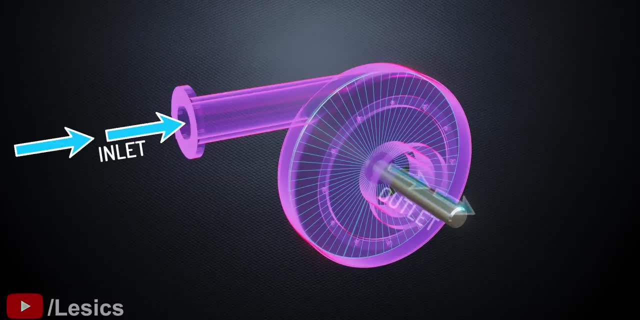 tangential to it. A provision for the fluid to exit is at the center of the turbine. Assume an inlet fluid with slightly higher pressure than the atmospheric pressure is entering the inlet nozzle at low speed. What do you think about the path this fluid takes? 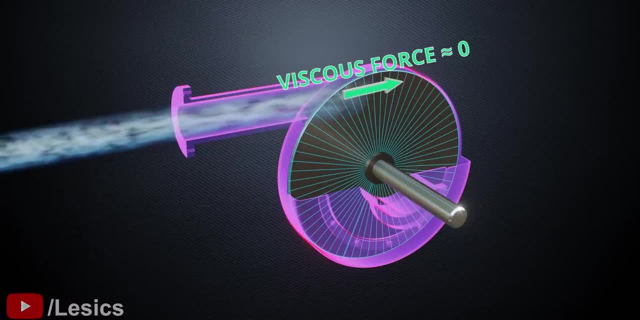 Since the fluid has a low velocity, the viscous force between the disc and the fluid will be very minimal and the disc won't rotate. The exit hole is at atmospheric pressure, which means the fluid will have a slightly higher pressure than the disk. The fluid will have a slightly higher pressure. 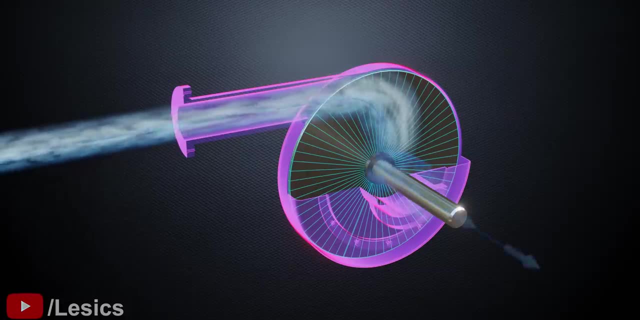 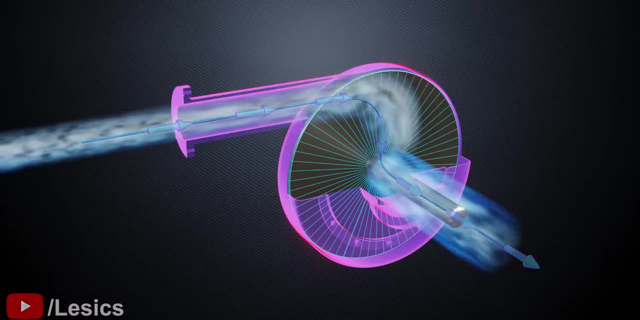 than the atmosphere and naturally flows towards the center almost in a straight line. Now let's increase the fluid's speed and see what happens Here. since the fluid has a greater speed, the interaction between the fluid and disc surface will produce sufficient viscous. 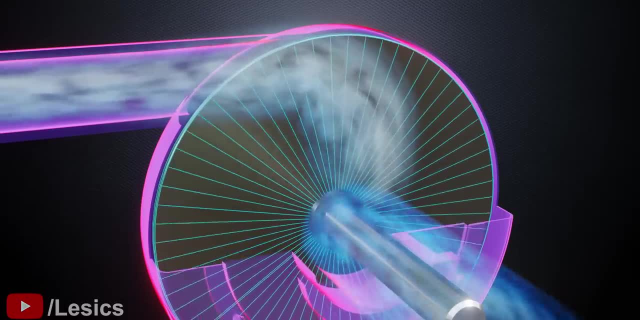 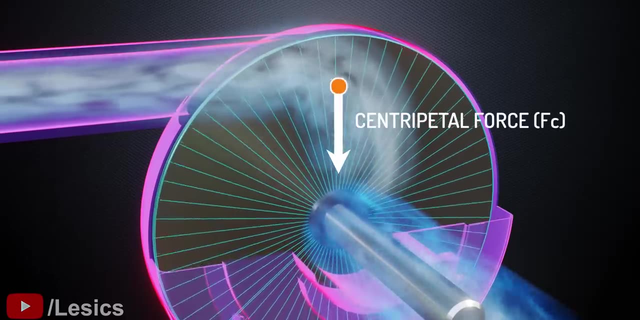 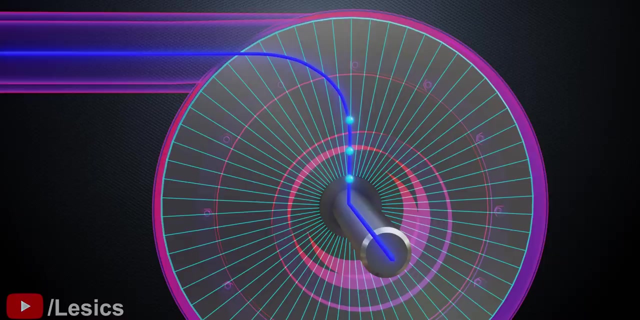 force to turn the disc. Here comes an interesting twist. When the fluid particles are rotating, they need a certain amount of centripetal force to maintain that motion. A fluid particle of the same velocity requires more centripetal force near the center than away from. 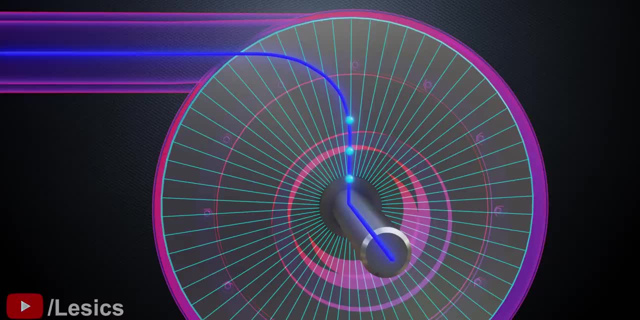 it. For this reason, the rotating fluid particles have a tendency to move away from the center. However, the turbine exit is at the center, so the fluid particles have to reach it eventually. Due to these opposing effects, in the rotating case the particle motion will curve out as shown. 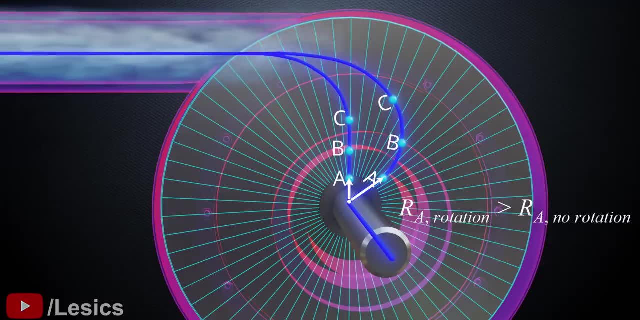 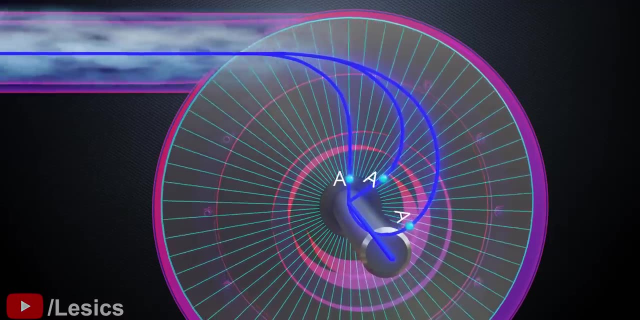 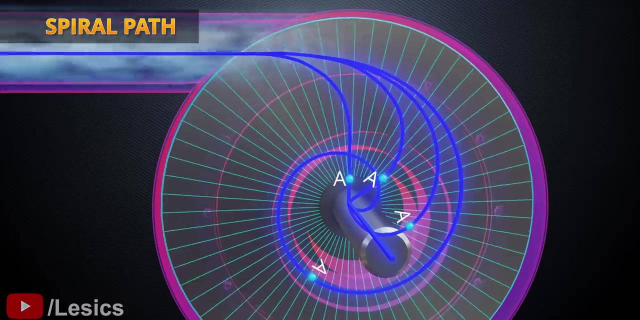 If you compare the radii of particle A in these two cases, clearly the curved path of the fluid particles have more radius. Now let's gradually increase the fluid speed. You can see the curvature of the fluid particles will further increase and form a kind of spiral. This concept is clearer when you track the 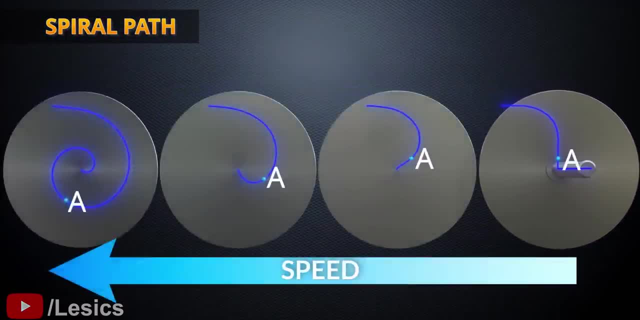 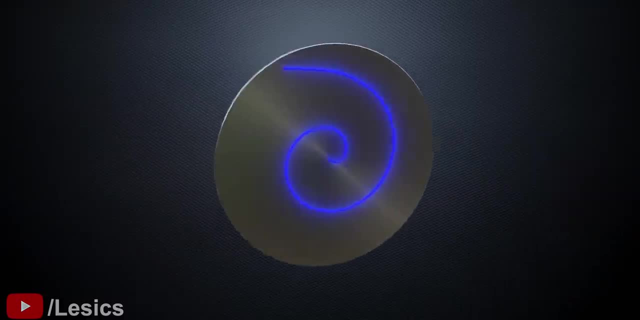 same fluid particle for different disc speeds. The greater the disc speed, the more the particle moves away from the center. The fluid flow's spiral shape is, in fact, a blessing in disguise. The spiral shape increases the contact area between the fluid particles and the disc. The contact area between the 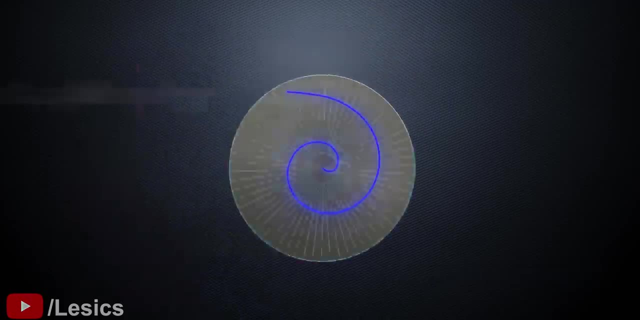 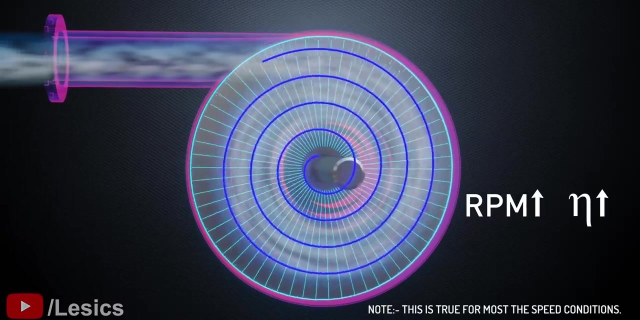 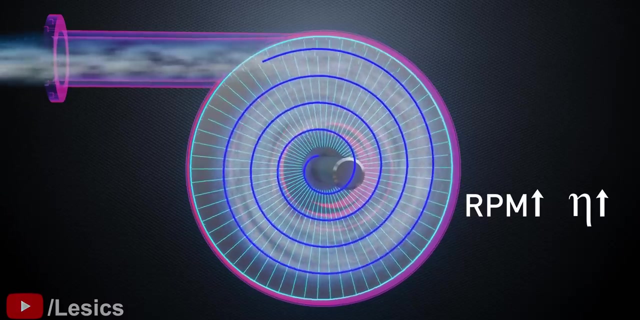 fluid particles and the disc surface, thus increasing the viscous force production on the disc. This effect also means that the faster the turbine rotates, the more energy it will extract from the fluid. In other words, the Tesla turbine exhibits high efficiency during high-speed. 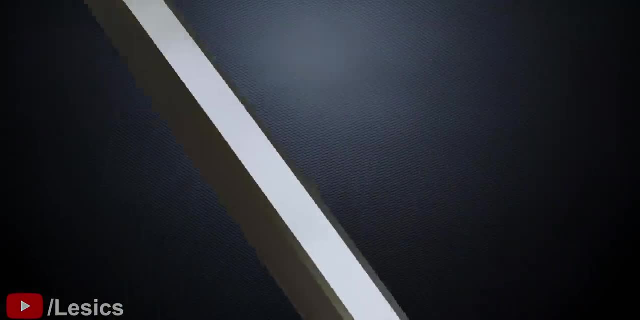 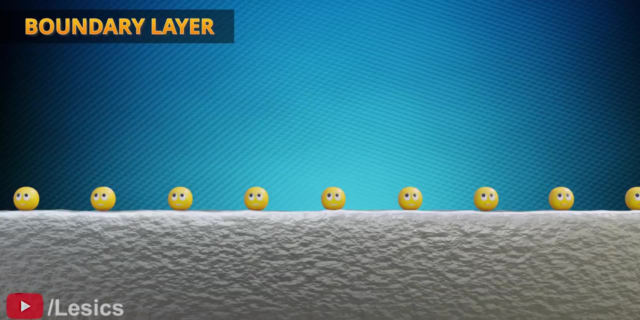 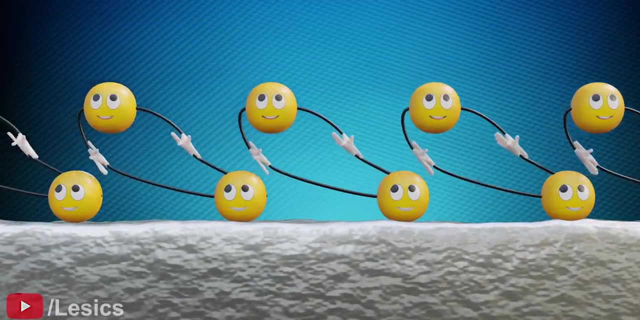 operations. To improve this design further, we need to understand a key concept called boundary layer thickness. We can observe in this system that the fluid particles which are in the center are in close contact with the disc, adhere to it and form a stationary layer. The next: 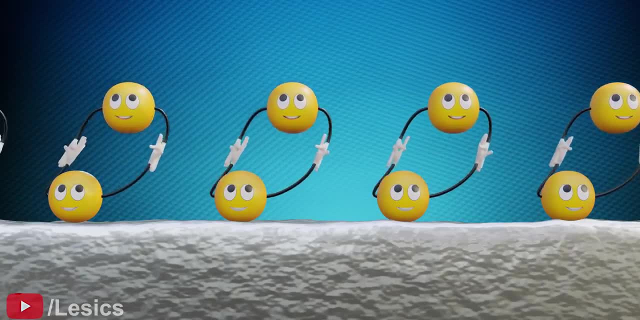 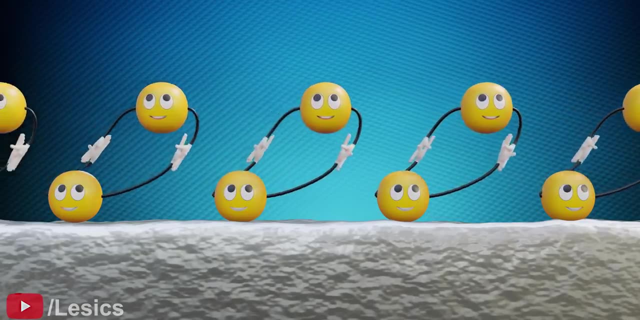 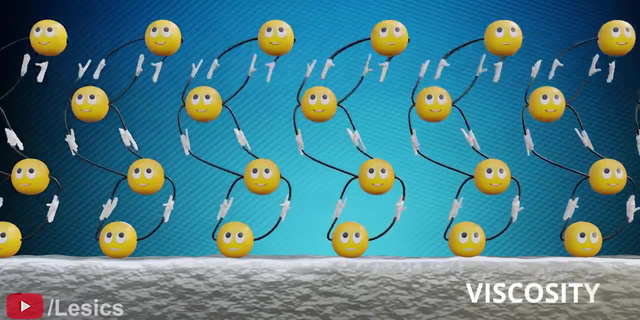 layer of molecules tries to pull the stationary layer in the flow direction. However, in this process they lose some energy to the stationary layer molecules. The same thing happens with subsequent layers. This tendency of fluid particles to resist the flow of the other particles is known as viscosity. In this way, you can clearly observe a velocity variation. 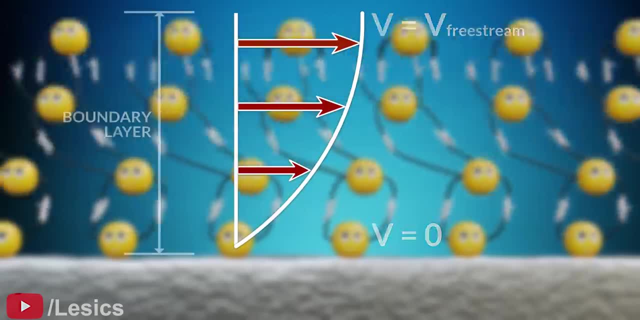 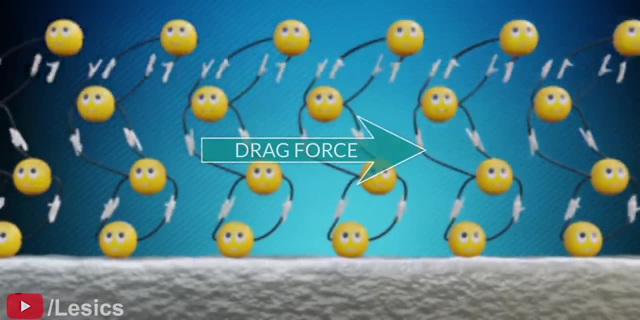 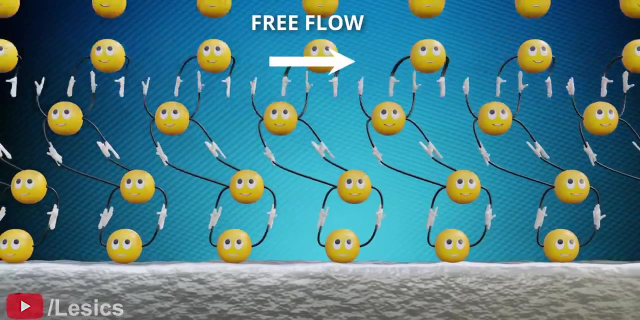 The region up to which this velocity variation exists is known as boundary layer region. Clearly, inside the boundary layer, one fluid layer produces a drag force on the neighboring layer, since a relative motion occurs between the layers. However, outside the boundary layer, 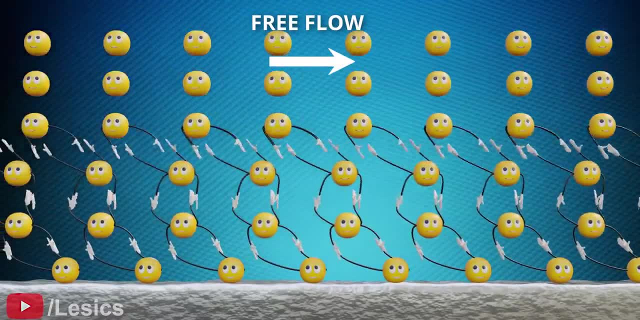 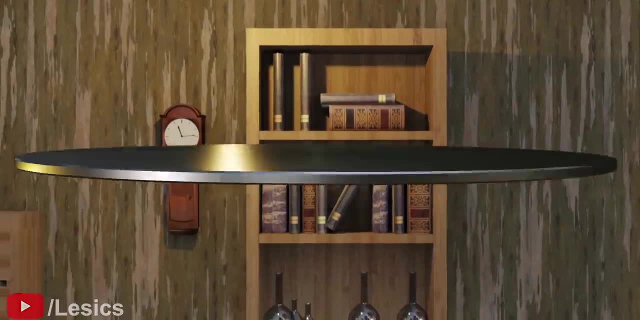 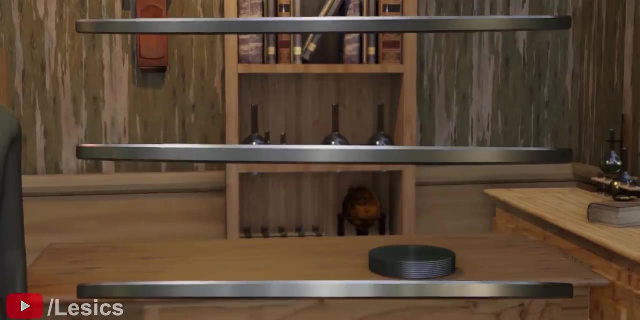 no relative motion occurs between the layers or the force between the layers is zero. To make use of this boundary layer phenomenon, Nikola Tesla came up with a unique idea: He added two more parallel disks. Now let's observe the flow: A boundary layer is formed on every surface. 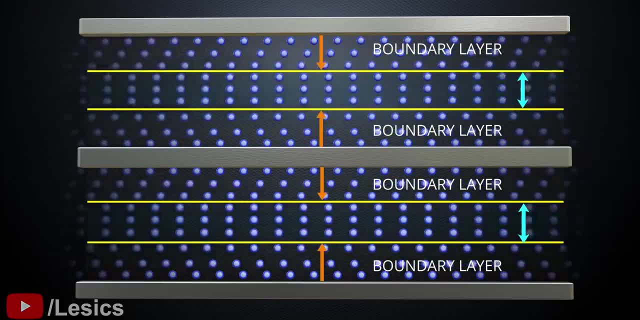 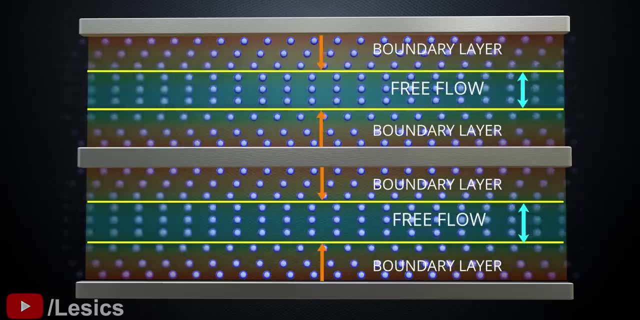 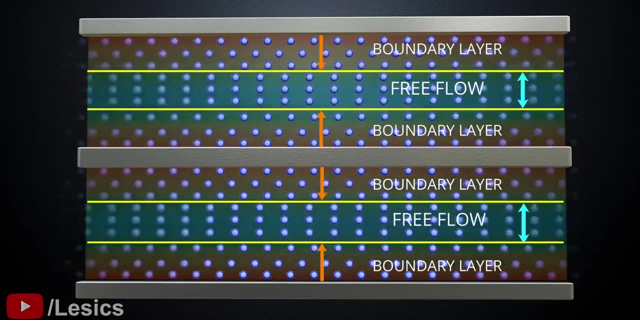 As we saw earlier, the particles in the boundary layer region will try to drag or rotate the respective disk. However, you can see a region outside both the boundary layers where fluid particles are flowing freely without any velocity gradient. This free flow does not impart any energy to the disk and contributes little to the 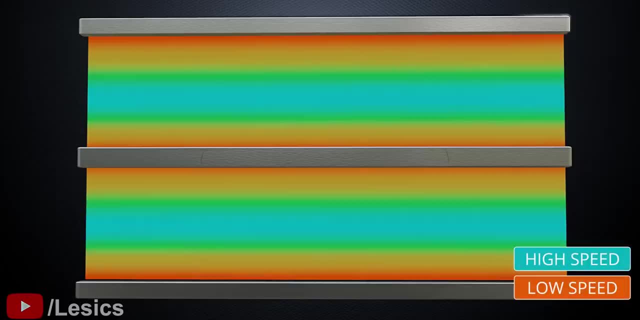 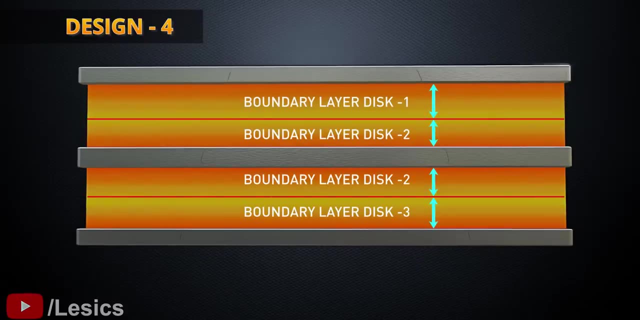 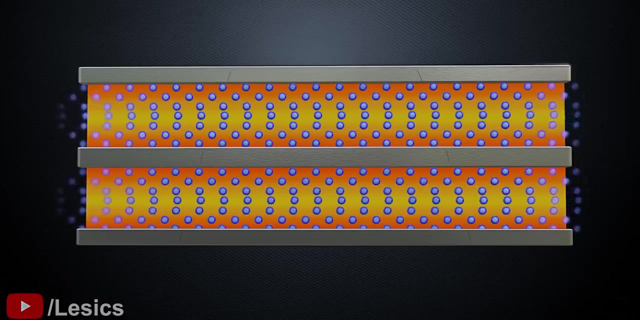 torque generation To make his turbine more efficient. Nikola Tesla brought the disks closer, keeping the gap approximately twice the boundary layer. Here no free flow occurs. The two boundary layer regions are touching each other and we can see the shear effects are now dominant in between the disk space. 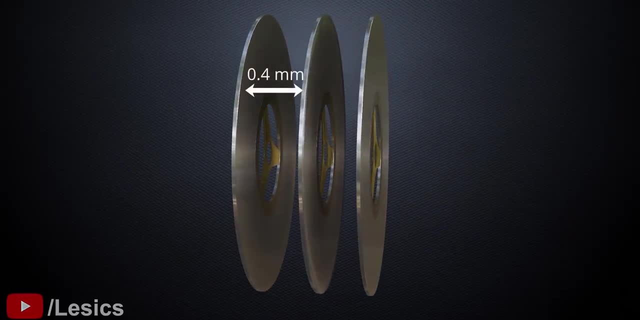 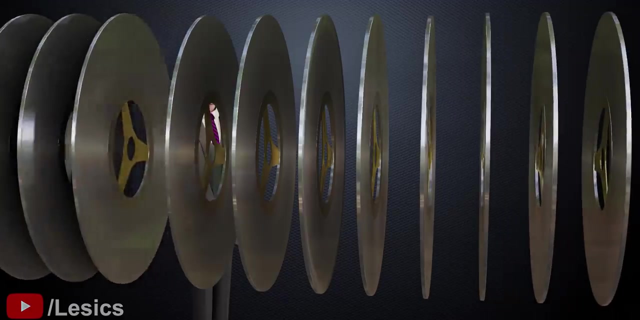 For steam. this ideal distance was fair. Nikola Tesla's turbine had a diameter of 0.4 mm and the diameter of the disk is 0.4 mm. Using this method, Tesla improved the torque output of his turbine. Tesla found that by increasing the effective area between disk and fluid, the turbine can 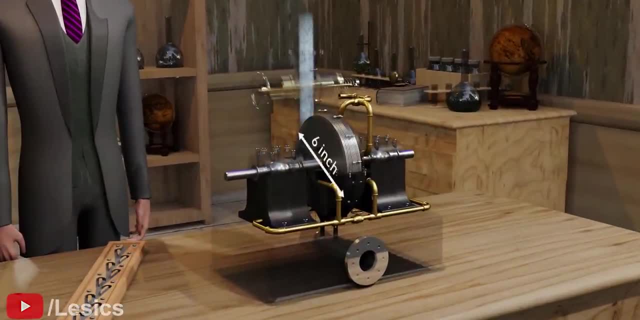 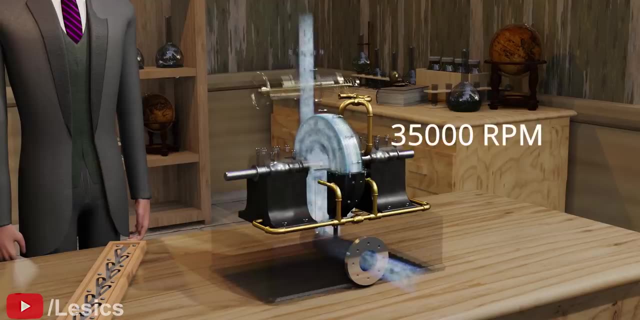 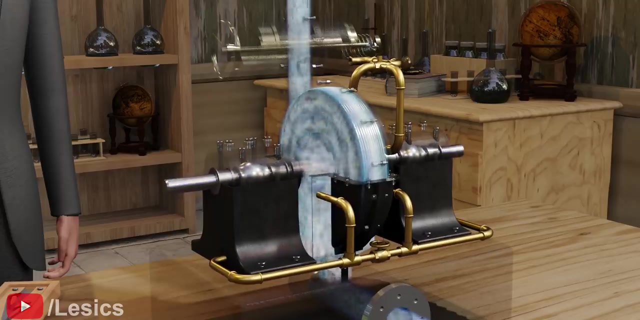 produce more torque, so he added more disks. This model had a diameter of 6 inches. However, this design failed horribly. The issue was that this turbine would run at a very high speed- 35,000 rpm. Tesla never thought that this turbine would produce such a high rpm and the disk strength. 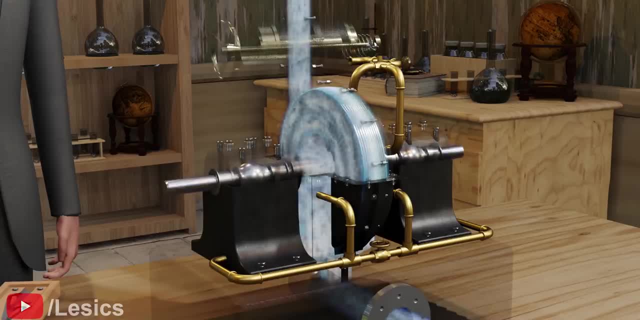 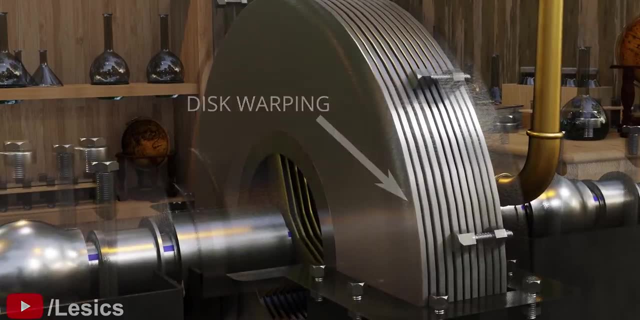 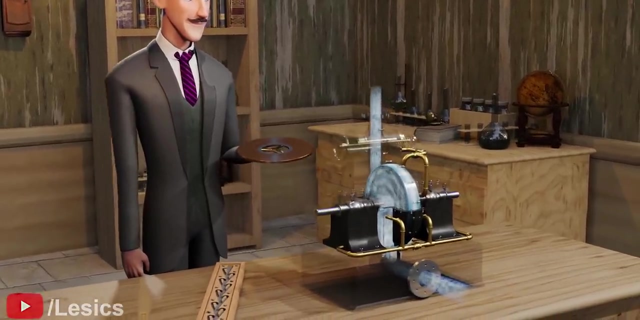 was not sufficient enough to withstand the huge centrifugal force produced in the material, resulting in material expansion and disk failure by warping. Nikola Tesla could not find any material to withstand such a high rpm at that time. Eventually, he had to reduce the rpm to less than 10,000 to save the disks from mechanical 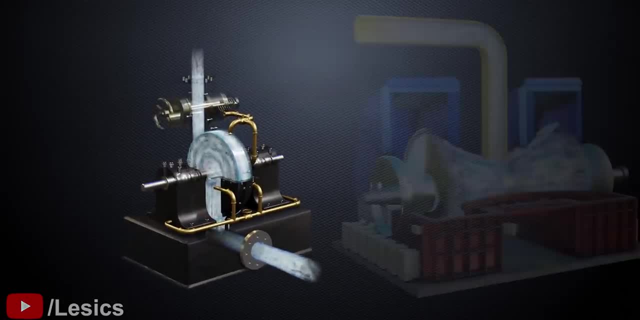 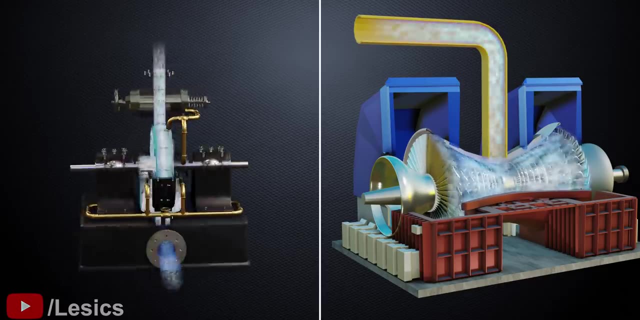 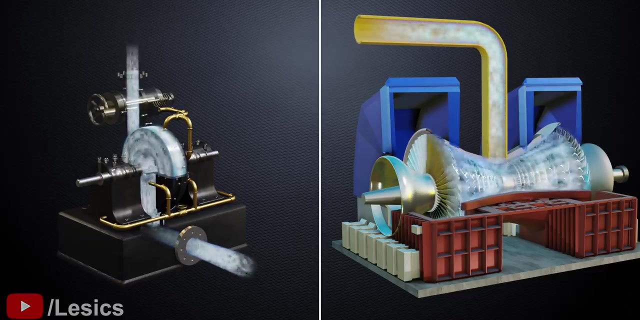 failure. Now for the big question: Despite the fact that Tesla turbines are so easy to construct, why aren't they used in the power generation industries? The reason is that the modern-day steam turbines are more than 90% efficient. We know that the Tesla turbine becomes more efficient as the rotor speed increases, but